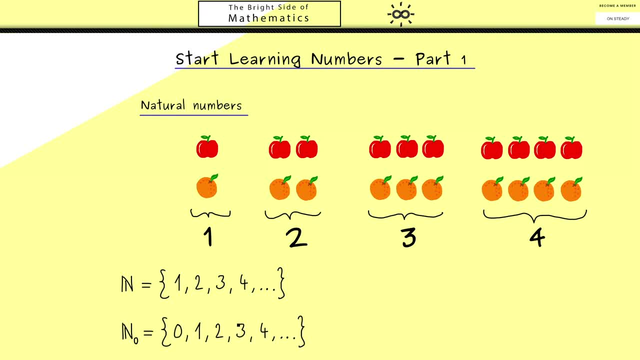 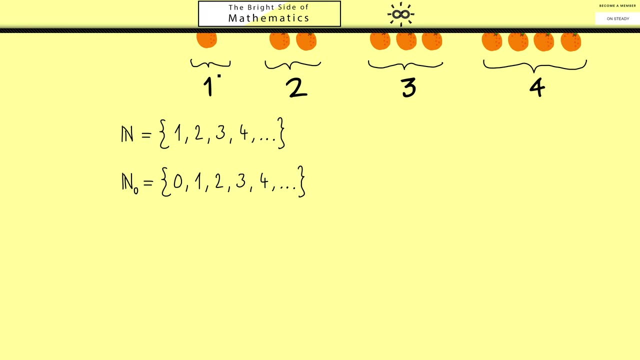 numbers that also include zero as a number. I will use the symbol n0 for this set, but be careful: often also n is used for this set here. Okay, with this, let's start constructing the natural numbers, As we have seen in our examples, with apples and oranges the size of a. 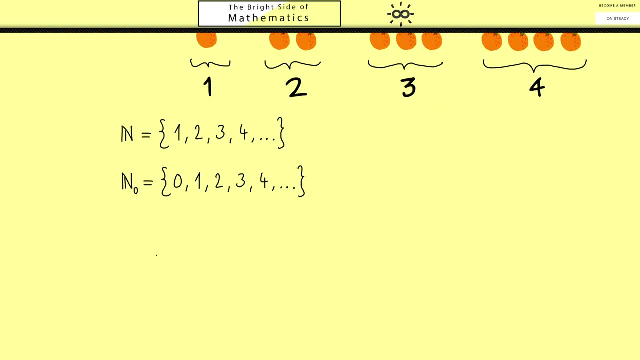 set can be used to define a number, And we already know one particular set, namely the empty set. By definition, the empty set does not have any elements, so it represents the number zero, And now it makes sense to use this as a definition for our new 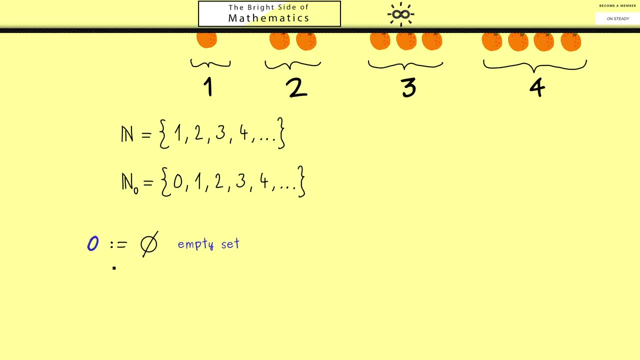 symbol zero. Maybe it looks a little bit strange here, but keep in mind we already have the set theory, so it makes sense that every new object we introduce should also be a set. We did the same thing when we introduced ordered pairs and maps. Now for the next step, for defining the number one as a set. we need a new set that contains: 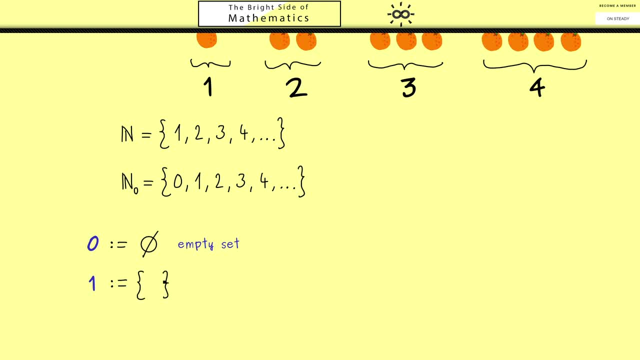 only one element. We could take any element we want, but the only thing that is defined yet is the empty set. So we put zero inside the set brackets and we get out a new set. What you should see is that what we do here is exactly the same thing we had in mind when 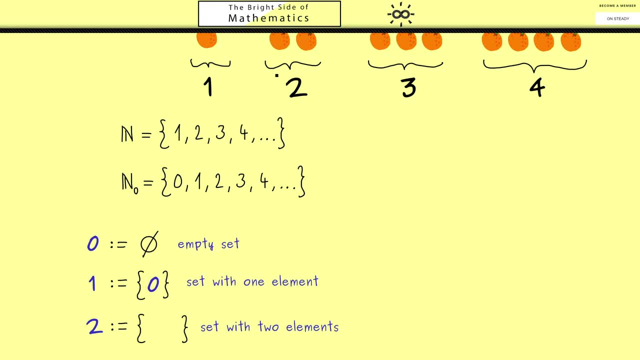 we dealt with the oranges. However, here we don't need any real world objects, we just need the abstract concepts in set theory. Ok, now for the number two. we need two elements. so what do we do? We take the only two elements we know. 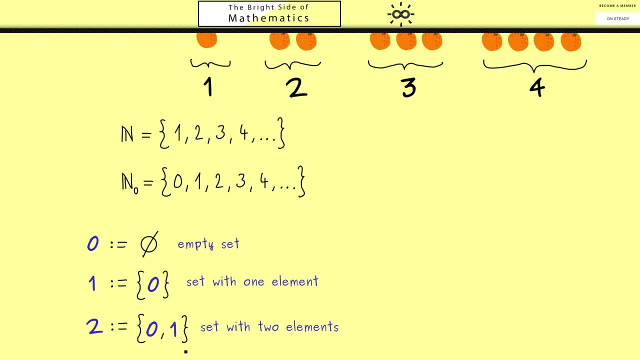 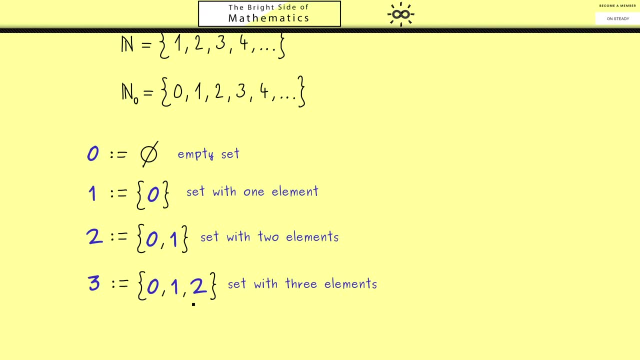 So zero and one, because we know they are different. At this point you should see how this game works and we can just continue it. Therefore, this is our number three as a set, and in the same way we can write down the number four. However, here you might already wish for a shorter way to write it down. 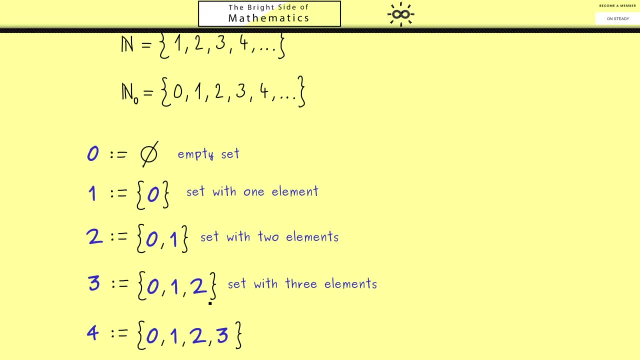 And, of course, if you compare to the set before, three we just add one element. For this reason we can just write it as a union. So this is what it is and maybe it looks again a little bit strange, but keep in mind three is a set here and here we have the set that contains three as an element. 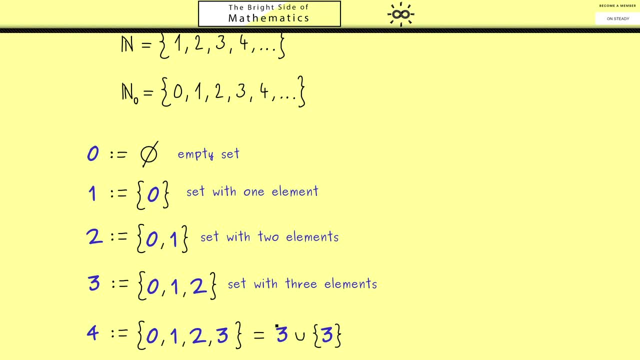 Ok, but with this formula, you now know how to construct the next number in a set. Ok, now we have the set that contains three as an element. Okay, but with this formula, you now know how to construct the next number in a set, And then we get all the numbers we want to have. 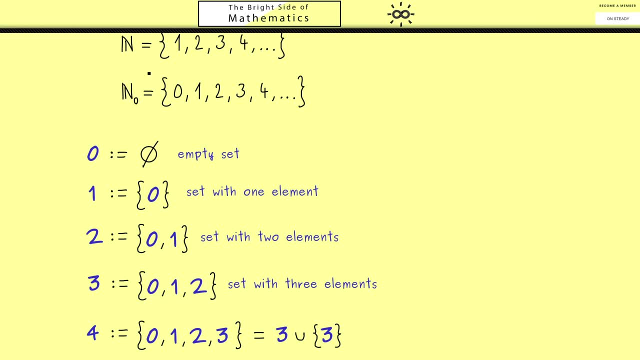 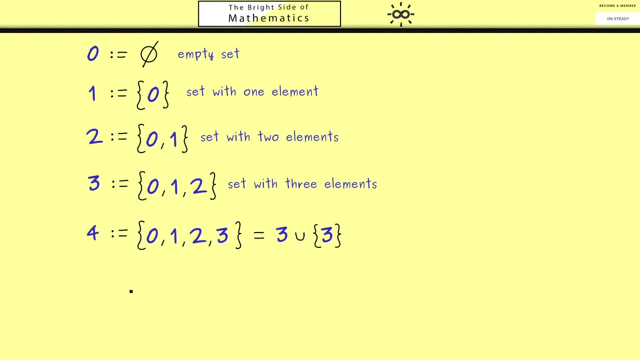 And after that we want to put them into one set and call it the natural numbers and zero. However, there you might see a problem, because this whole construction here never stops. Or to put it in other words, the natural numbers, the set and zero should have infinitely many. 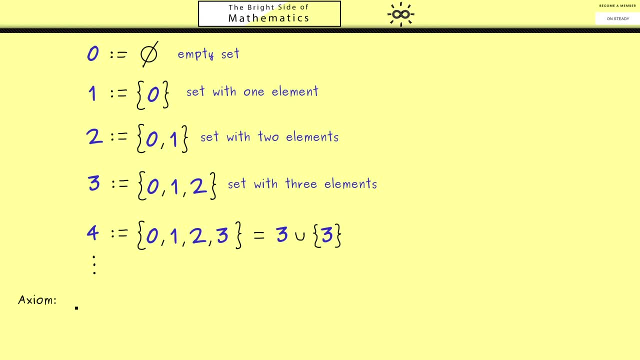 elements, And that is something we have to put into our set theory. so we call it an axiom. It is simply something we put as a true statement into our theory. For example, the existence of the empty set was also an axiom we put into the set theory. 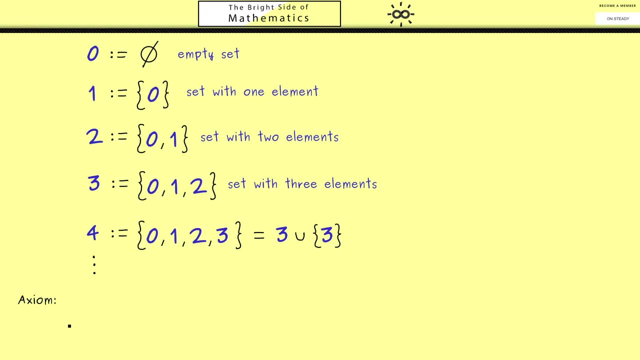 And now we want to put in the existence of the natural numbers. So we say there is a set and zero with the following two properties: The first one is that we have a starting point at zero, so the set zero lies in n zero. And the second one tells us that for all numbers, 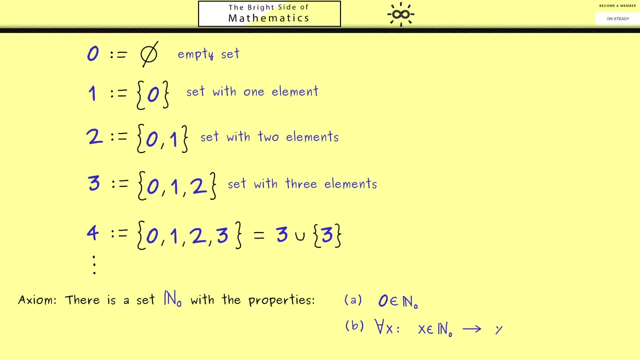 in n0. also, the successor lies in n0. And now we know we can write it as this set here. As a reminder, here we have the conditional from logic and i already told you sometimes it's written with a doubled arrow. Later we will also do this, just to avoid confusion with the arrow. 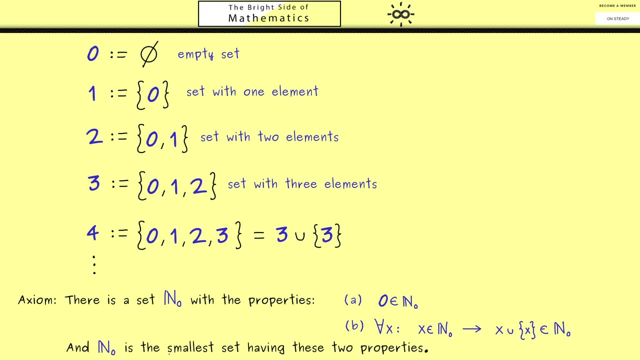 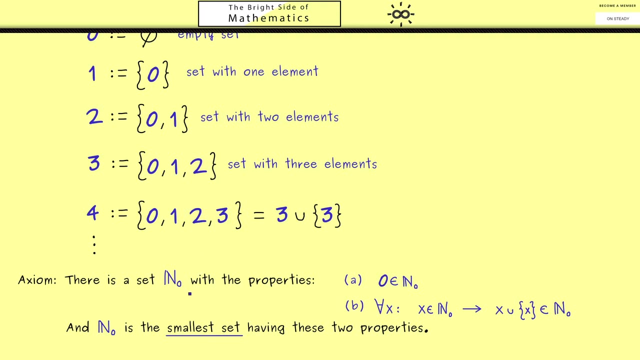 from maps. However, to finish our axiom here, we also have to say that n0 is the smallest set that has these properties. This simply means that any other set with these two properties is a superset of n0.. Okay, and with this we finally have the natural numbers in our set theory. 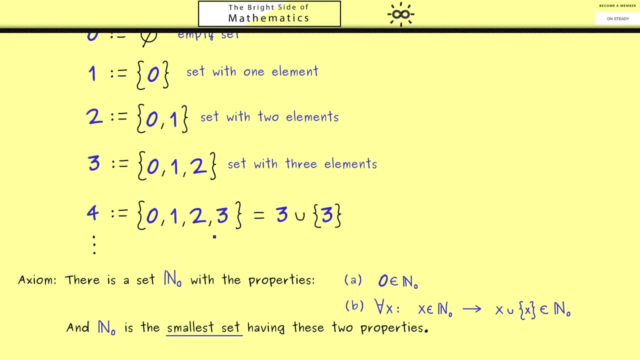 It's constructed with sets. it has sets as elements such that we can work with it. That's how you should see it. It's not the explanation of numbers. it's a working tool for us. Therefore, it's often called a model for the natural numbers. Now, with the natural numbers. 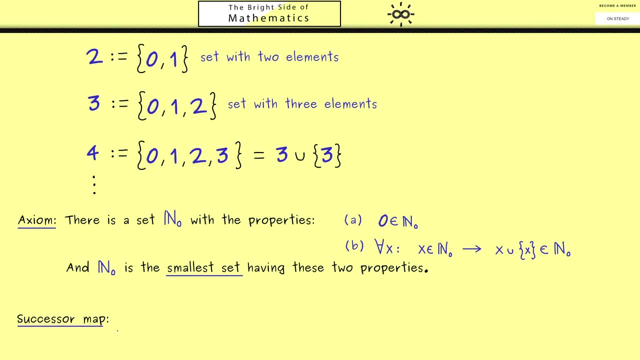 we immediately get a map, we call the successor map, We denote it with s and it goes from n0 into n0. And the definition we already know. we send the number x to the union Because we learned this gives us the successor. For example, if we put the number 6 into the map, we get out the number 7.. 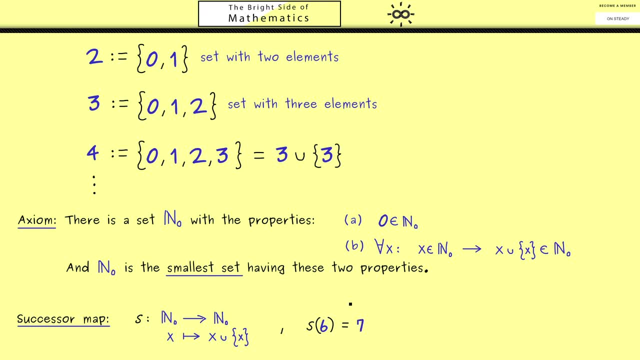 Okay, i think that's good enough for an introduction. In the next video we will talk about all the properties of the natural numbers and all the properties of the numbers, Also how we can define the addition. So i hope i see you there and have a nice day. Bye. Thanks for watching. 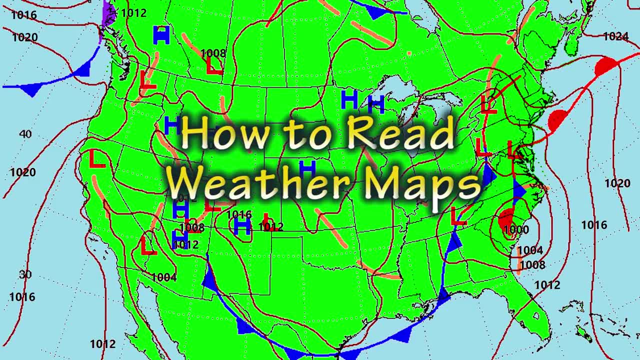 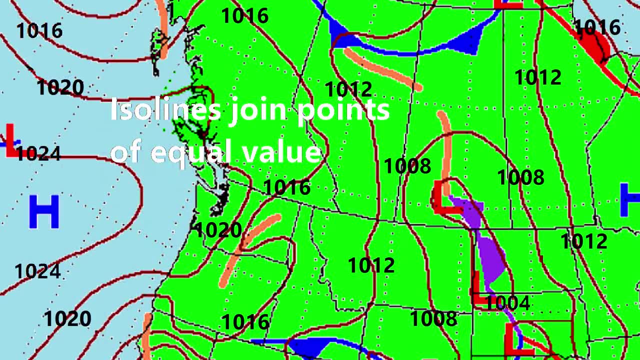 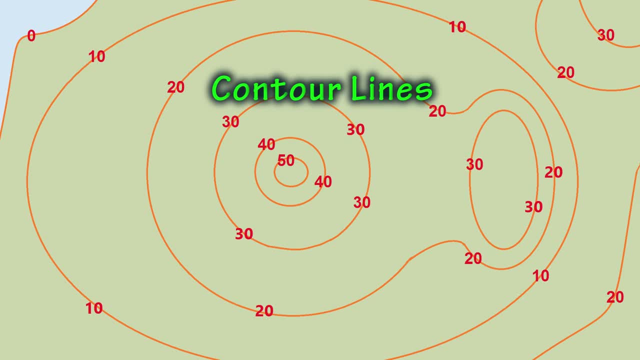 Weather maps, also known as the synoptic chart, are an example of an isoline map. Isoline maps are made up of lines that join points of equal value. Contour lines drawn on a topographic map are another example of an isoline map. 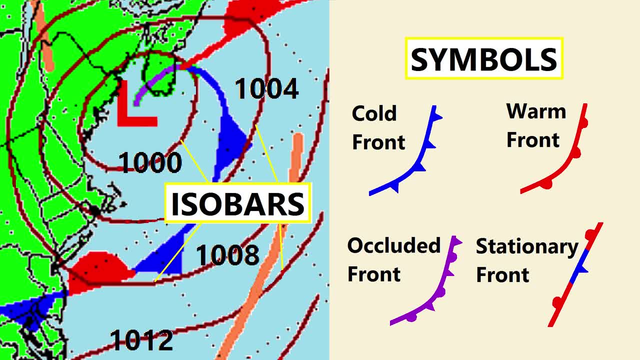 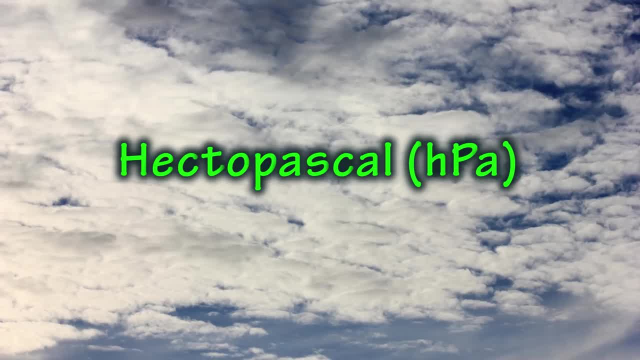 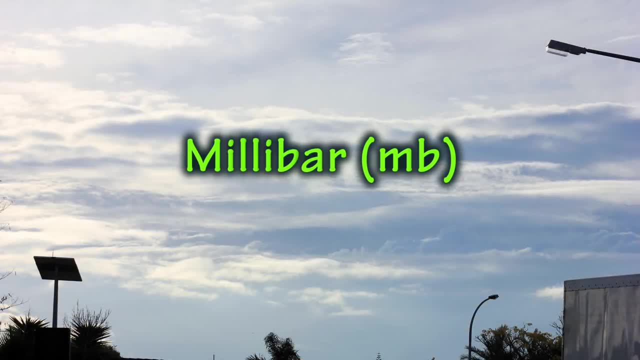 Weather maps use lines called isobars plus other symbols to join together lines of equal air pressure. Today most meteorologists use the hectopascal for measuring atmospheric pressure. Many weather reports to the public use the millibar. One hectopascal equals one millibar. 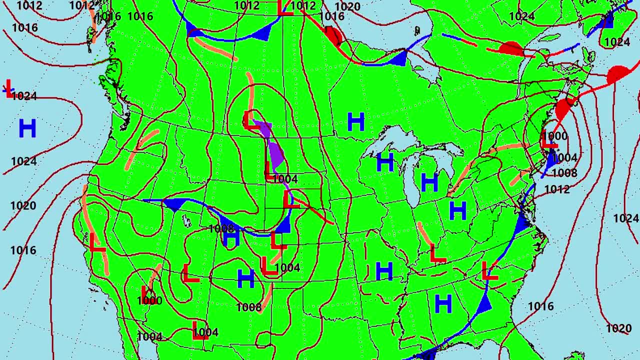 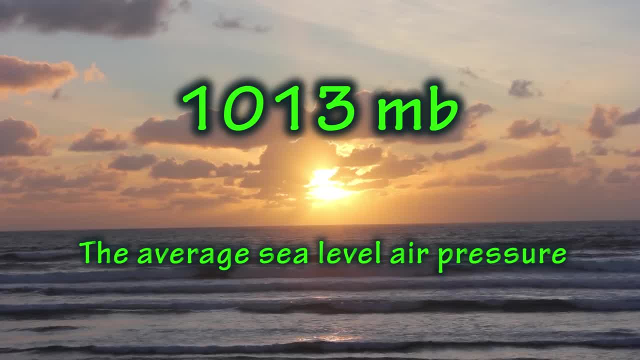 On these American weather maps, the isobars are drawn at intervals of four millibars. 1,013 millibars is the average sea level air pressure. Therefore, areas with an air pressure of 1,013 millibars are drawn at intervals of 4 millibars. 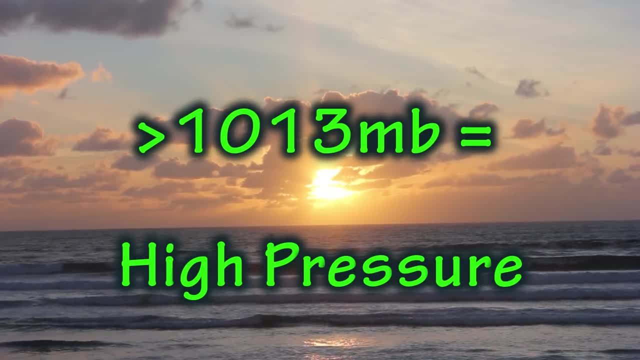 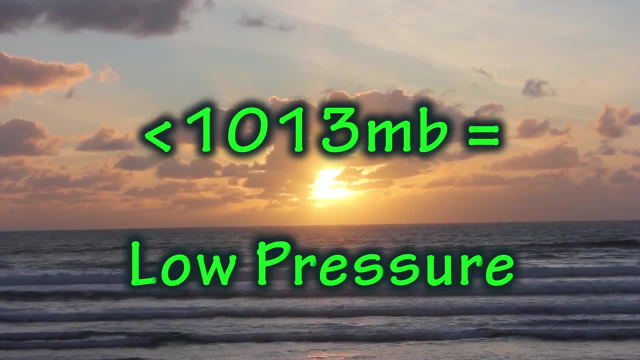 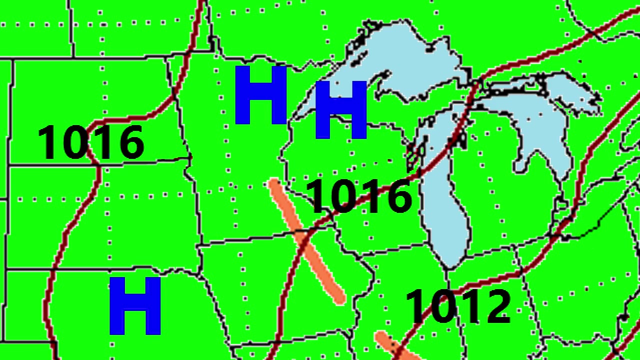 The areas with an air pressure of over 1,013 millibars are considered to be areas of high pressure, and areas with an air pressure below 1,013 millibars are considered to be areas of low pressure. On a weather map, areas of high pressure or anticyclones are identified by a letter H.